The wolves' absence and reintroduction changed Yellowstone in large and often surprising ways. It all comes down to how the rivers flow. For one thing, wolves prey on elk and the elk know it, So their behavior changes when wolves are in the area. Elk are generally nomadic, staying on the move as they munch on plants, But without any wolves around. the elk became much less cautious, preferring to settle down and eat a lot in one place at a time. The elk even ate all the way down to the riverbank, somewhere they wouldn't dare linger if there. 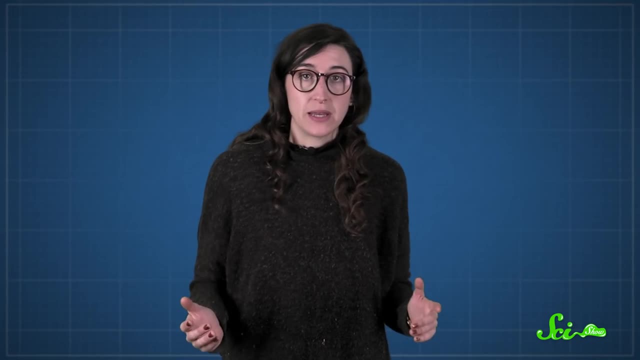 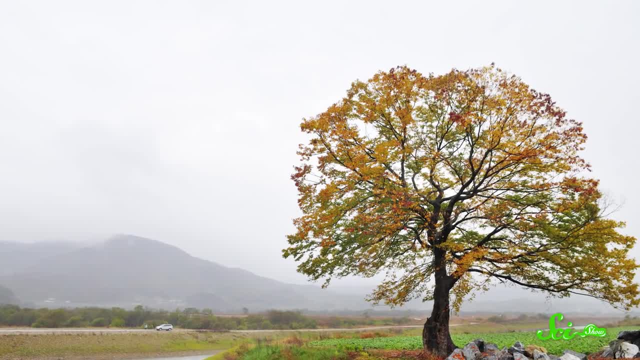 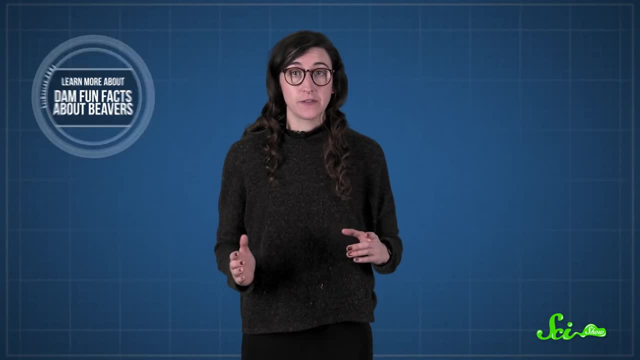 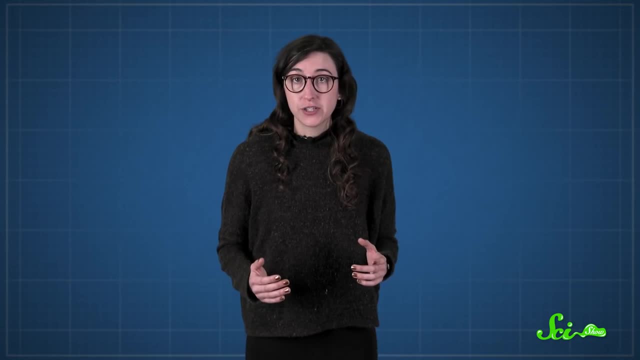 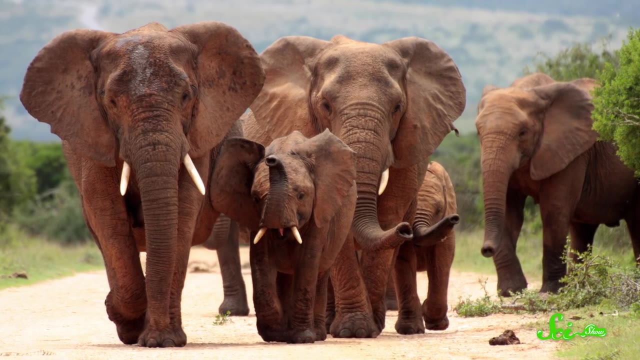 of wolves has resonated throughout Yellowstone, And research into other wolf habitats will help work out what's unique to Yellowstone and what can be applied elsewhere. Elephants also do a lot to manage their environment, from what goes on in their mouths to what comes out the other way. 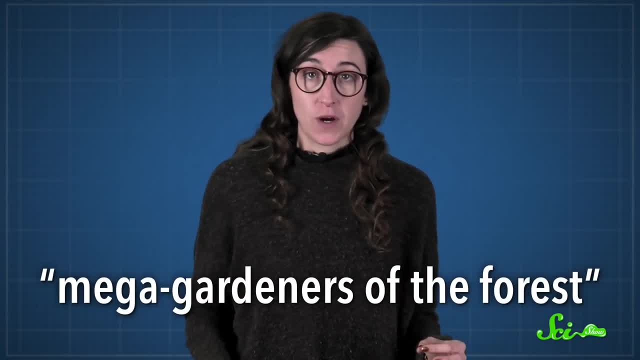 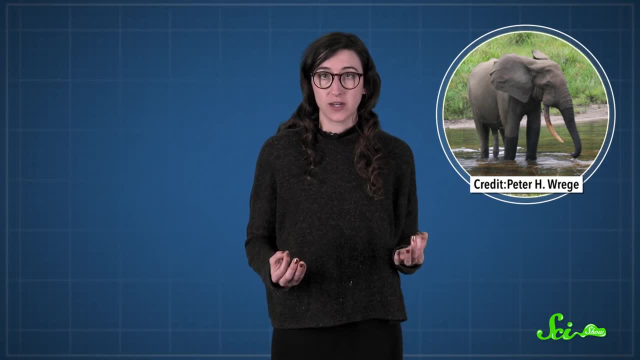 They're sometimes known as the mega-gardeners of the forest. For example, without African forest elephants, a single species of acacia tree tends to dominate African forests. It grows fast and shuts out the light from other plants, And the elephants help counter that. 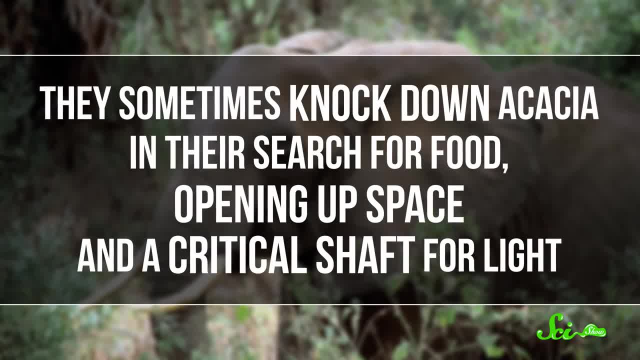 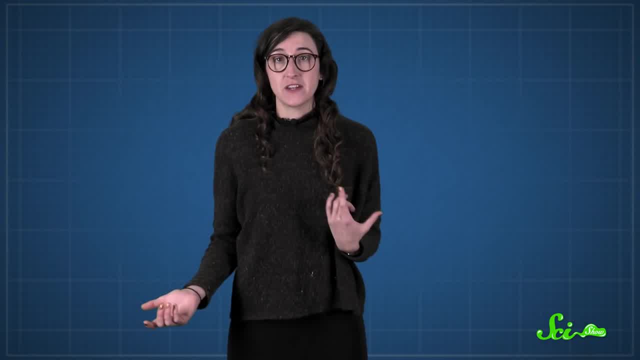 They sometimes knock down acacia in their search for food, opening up space and a critical shaft for light. Other plant species seize their chance, adding to the forest's biodiversity. The smaller branches that they knock down provide hidey holes for lizards, which are more diverse in places like Yellowstone. This is where elephants roam. When reaching for leaves or fruit, they'll often knock off a bunch more, And these windfalls get picked up by smaller ground-dwellers like warthogs, as well as. the kudu, which is a type of antelope. All this eating results in plenty of dung- around a metric ton every week, And all that poop becomes a mini-ecosystem all by itself, since it's rich in nutrients that the elephants couldn't process. 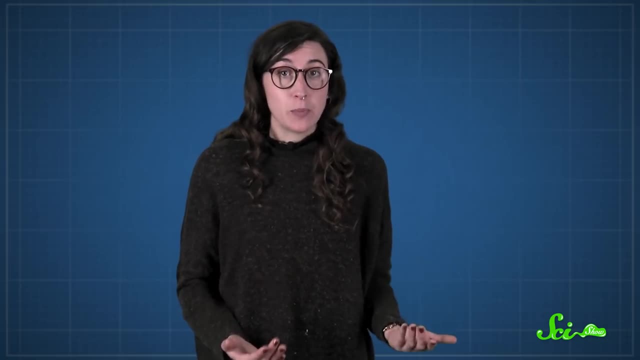 Fungi live in it, as do insects like beetle, larvae, crickets and spiders. In 2009,, three species of frogs were found, happily living in Yellowstone. The first species of frogs were found in Yellowstone. The second species of frogs were found in Yellowstone. The third species of frogs were found in Yellowstone. The fourth species of frogs were found in Yellowstone. The fifth species of frogs were found in Yellowstone. The sixth species of frogs were found in Yellowstone. And, of course, it's excellent fertilizer. Many plant species grow better in elephant dung than in poop from any other animal. 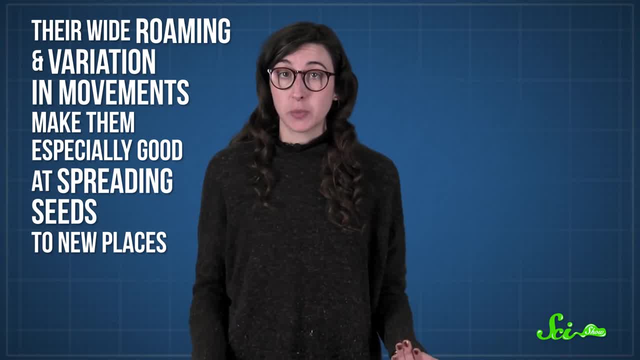 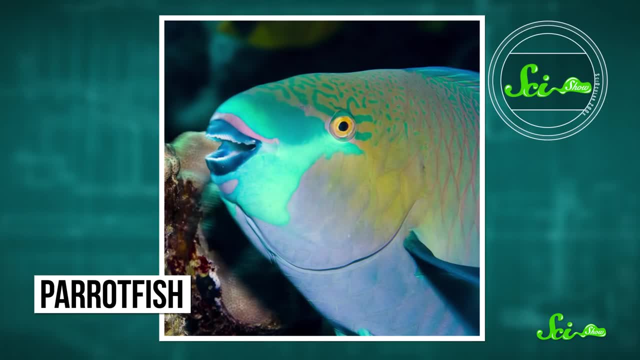 Their wide roaming and variation in movement make them especially good at spreading seeds to new places. But you don't have to be as big as an elephant to have a jumbo-sized impact on your ecosystem. Parrotfish are named for their tough, almost beak-like mouthparts.